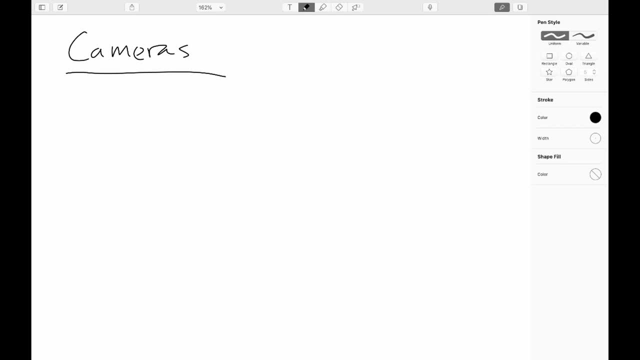 And for the most part this is the case here. So we'll start with a camera and then we'll scaffold our way up to thinking about the eye. So I'll think about a camera system that just has a single lens, Like so. 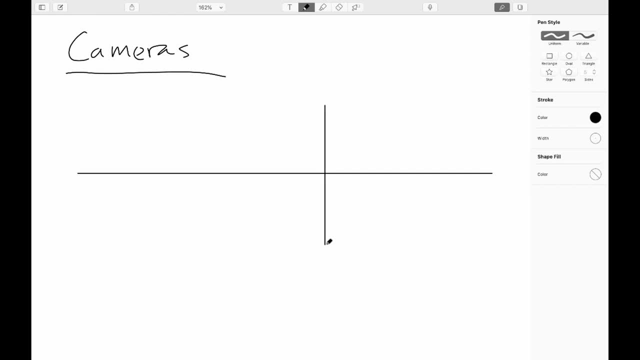 Oops, There we go Now. Now, In practice, real-world camera lenses, lens systems almost always have multiple lenses. This is to deal with an effect called chromatic aberration that we'll run into later. But we can go and take a look at it here and say, all right, usually you're going to have a relatively short focal length. 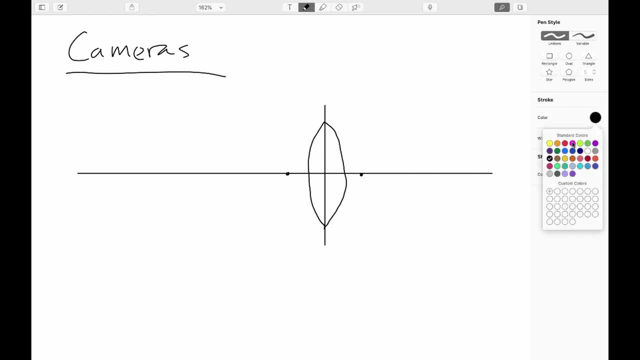 And with a camera you're going to have what's called the image plane of the camera, Somewhere a little bit behind the focal length. So if I go and look at some distant object, Let's say Way out here, There will only be one exact distance where this distant, where a distant object would come into perfect focus on the image plane. 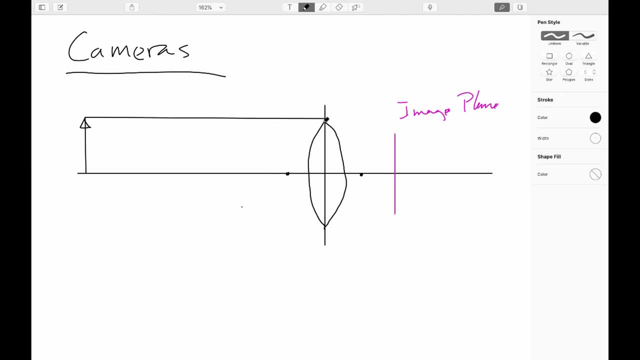 So let's just go ahead and locate it here, Oops, and I guess I'll have to move my image plane. there we go So, and I could draw a zillion more rays. I won't at the moment, Actually, I will. 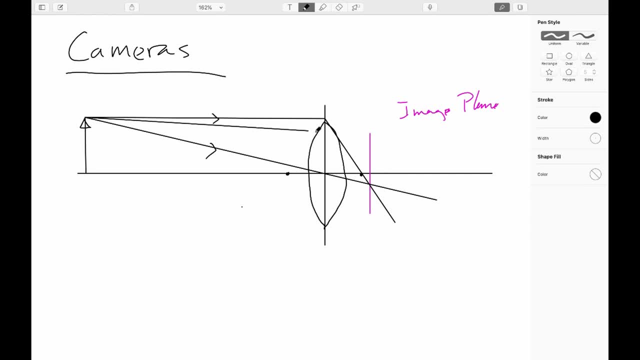 So I drew two of the special rays, but there's nothing to keep me from drawing a whole bunch more rays that would all be going through to make my image And if I happen to be at that one special location, everything's going to come into. 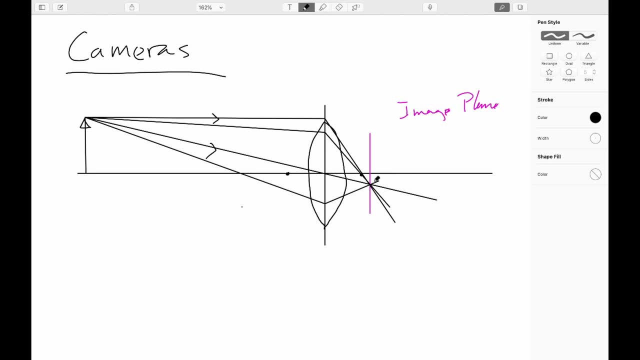 very sharp focus. But what would happen if you were literally anywhere else, if your object was anywhere else? Well, if that was the case, then the issue here is that these rays would not come to sharp focus, but you can see that they would be typically coming together kind of close. 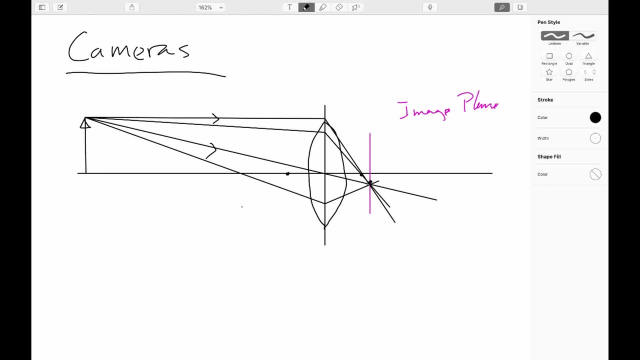 So how sharp is sharp enough? Well, On modern cameras the image plane usually has what's called a charge coupled device array or CCD array, And as long as all those cones make a blur that is smaller than a pixel on the sensor, then that's just as sharp as anything else. 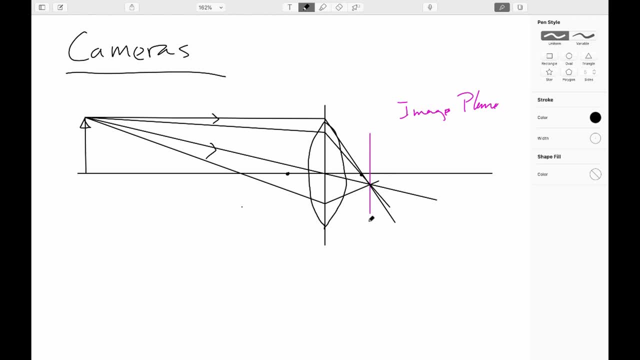 Okay, So usually what camera manufacturers will do is they will characterize this with something called the F number of the lens, And this is the focal length of the lens over its effective diameter, which could be the actual physical diameter. The focal length of the lens. is the focal length of the lens or a camera manufacturer? 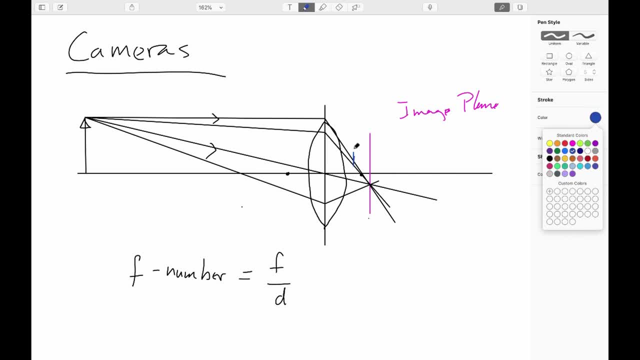 might decide to go stick some mechanical iris in in order to cut off some of the rays that are going in. By doing that, they'll make the cone of rays coming in narrower. By making it narrower you'll increase the extra distance. 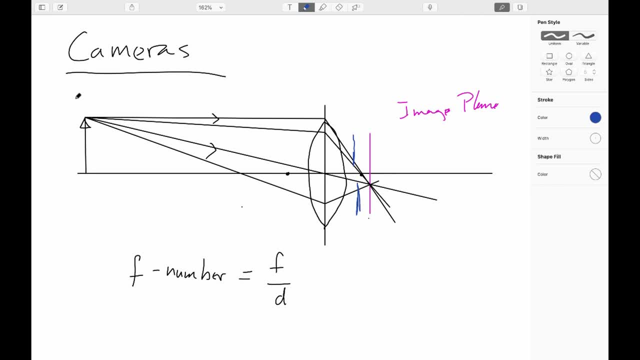 Okay, So that's what we're going to do, And then we're going to go back and forth. We're going to make sure that objects could be back and forth in front, be around the one perfect distance and still have an acceptably sharp focus, because it's all on the, the blur. 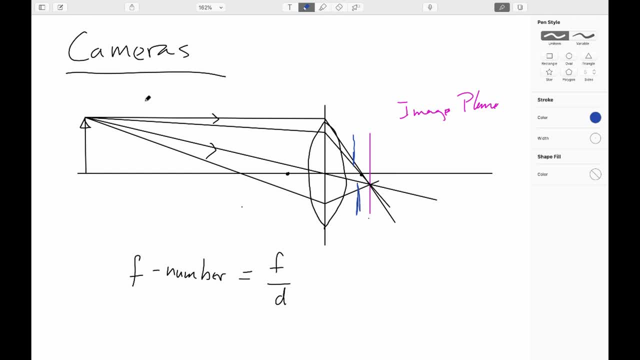 is the size of the CCD pixel or less. So from a sharpness perspective, the higher the F number, the better. Okay, It's saying that the diameter of the pencil is small and the eyes have to say compared to what the natural point of comparison is, the focal length. 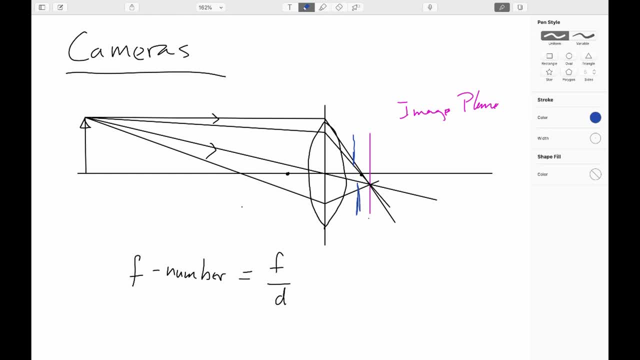 Now what if you decide that what you're taking a picture of isn't acceptably sharp? how do you adjust for that? Well, in a camera, the way that gets adjusted, The Carry Julie is supposed be the camera of theouch. 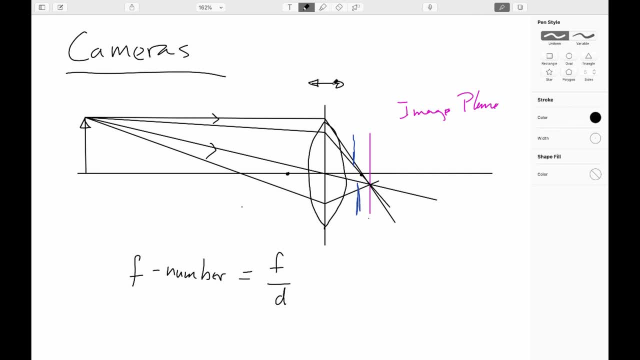 is you usually mechanically move the lens back and forth in order to bring it into focus. Now, one other thing about this F number thing that I'm mentioning, too- is you can also bring more and more things into focus, increase what photographers call the depth of field. 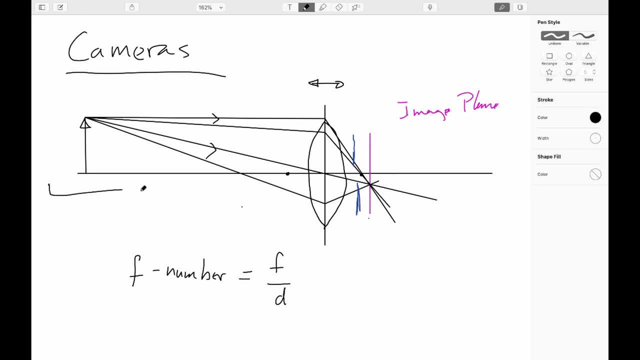 increasing the distance around the object where things are acceptably sharp, by making the mechanical iris ever smaller. However, if you do that, every time you cut the iris down, its diameter down by a factor of two, you've reduced the amount of light that hits the image plane by a factor of four. 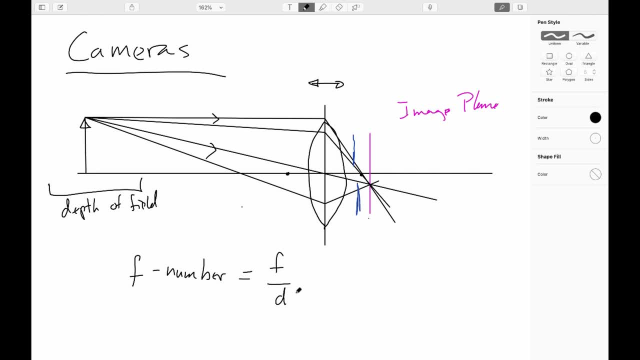 because the light passes, because what counts is the area of the aperture. So this is why in cameras you'll see, usually the F stops on a lens are marked in increments of F numbers that change by a factor of the square root of two. 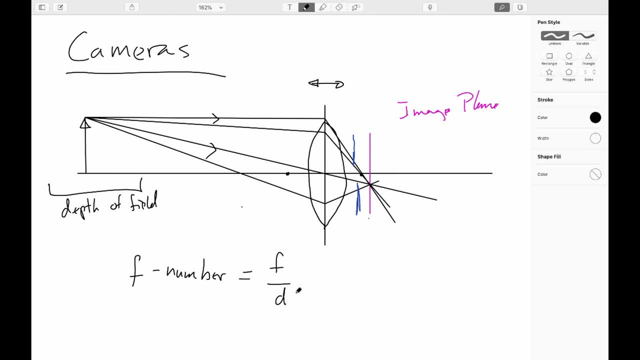 And this is so that each click doubles or halves, halves the amount of light striking the plane, the image plane Now, with modern digital cameras, there's a third thing that you can put in, which is called the ISO of the lens. 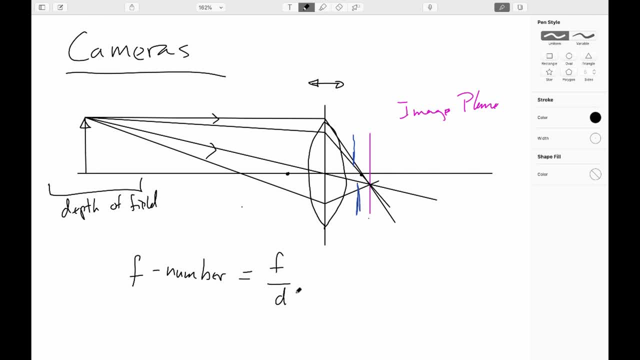 So you can increase the ISO, which is the sensitivity of the CCD array. You can make it. You can make it more and more sensitive, but at the cost of introducing electrical noise into the image. The other way you can get collect more light is just playing to have a longer shutter speed. 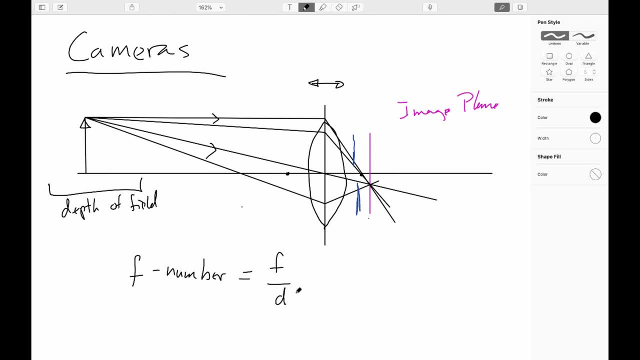 So photographers will play with these different choices of ISO setting, shutter speed and F number of the lens to get whatever desired effect they want. Okay, so that's the camera. So now let's go and look at an eye. And I'm just going to apologize right now and say that I am in no way, shape or form, a medical illustrator. 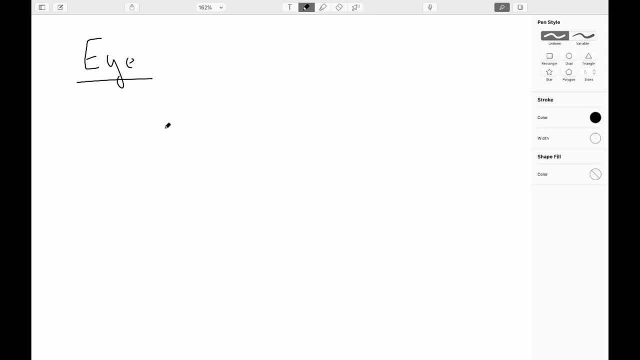 So, don't you know, just putting that out there. So, So the eye is spherical-ish. I'm going to put a little bump right out here. So this bump right here gets called the cornea of the eye, And then immediately- oops, immediately- adjacent to the cornea. 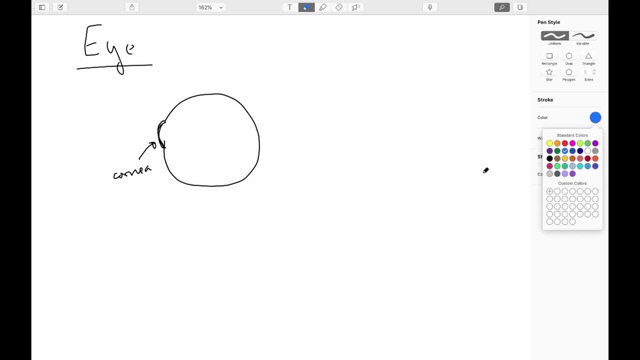 is a different medium called the aqueous humor, And that should be kind of flat there. if I can draw it a little better, There we go. That would be the aqueous humor A-Q-U. Aqueous A-Q-U. 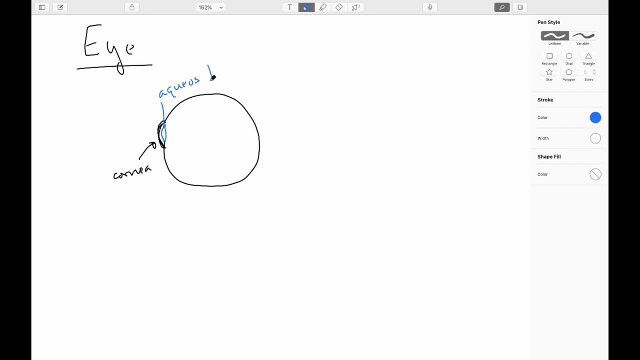 A-Q-U-E-O-U-S. Then behind that is the iris of the eye. Okay, Um, Let's look at that, Let's look at that And we'll draw that in, like so. Then, immediately behind that, is the lens of the eye. 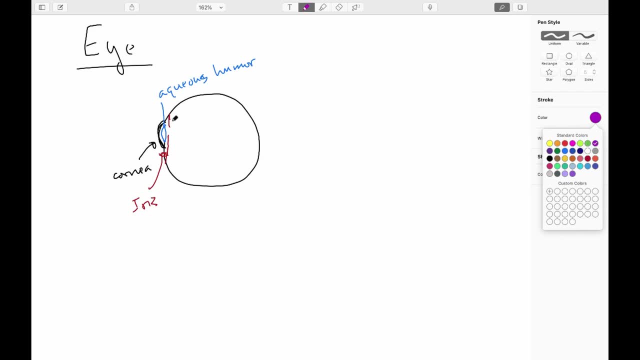 Let's see what color we'll do: Purple for the lens And again sort of misshapen a bit Like that. Then attach that to the eye, Attach to the lens are the ciliary muscles. What the ciliary muscle will do is it will flatten up the lens upon contraction. 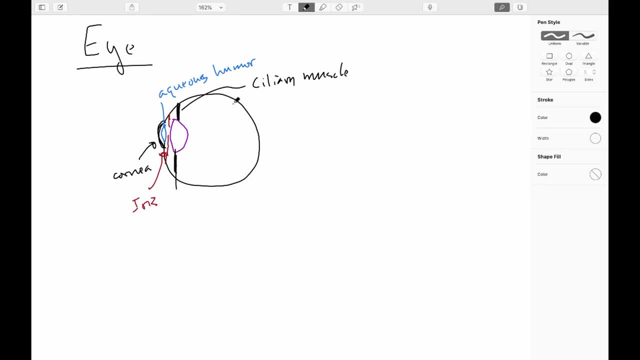 Then, at the back side to the eye, it will flatten up the lens, Then it will flatten the lens again. See, This isn't a ciliary muscle, This is a retina muscle. This is the retina. Can you see? the retina is the optic nerve. 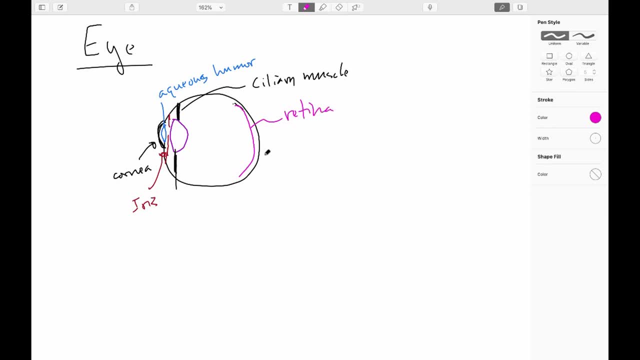 The retina is part of the pectoral muscles, It's the optic nerve. The retina is part of the eye And it's the optic nerve And also it's the optic nerve. I'll talk about the retina a little bit later. 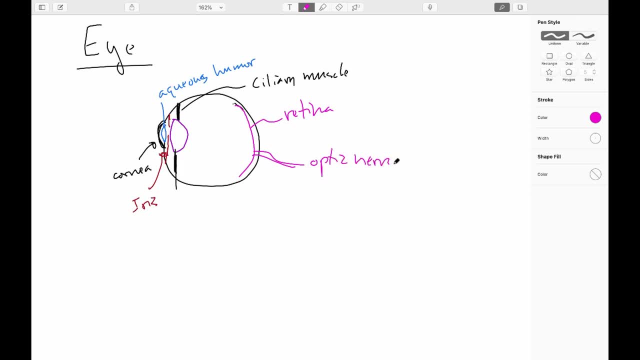 The optic nerve is part of the eye And I'll get back to uh the retina And to uh collect the image. you have the retina of the eye And attached to the retina is the optic nerve. The retina is an amazing complex. 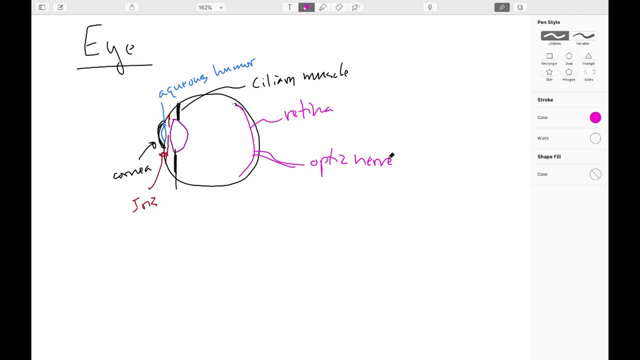 It uses photo collection of different photochemical sites, and it's amazing to see like this is really complex This collection of different photochemical sensors: typically one set of what are called rods, which are very sensitive but only give black and white information, and at least two different sets of what are called cones, although there are different species where there's more than two sets, but for humans two is typical. 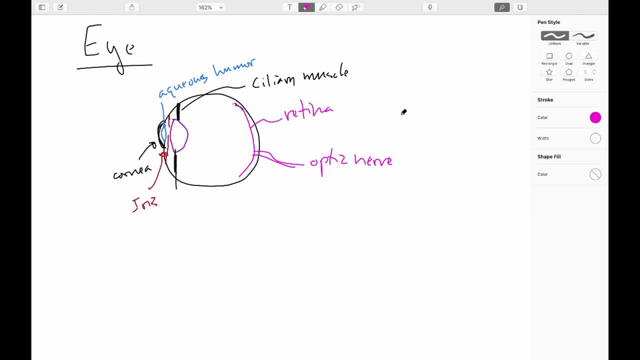 that provide color information, although they require a much brighter signal to give that. The density of these receptors is much greater in the center of the retina and much less out at the edges. Now you had the same issue: How do you bring an image to focus on the retina? 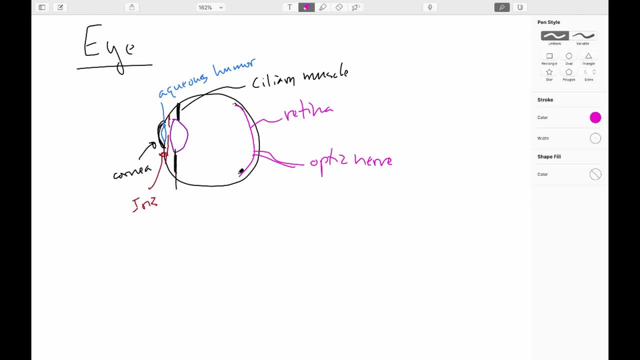 And this is done through what's called accommodation In the eye. you don't move the lens back and forth. Instead, what you do is you use the ciliary muscles to flatten the lens or, if it relaxes, then make it wider. 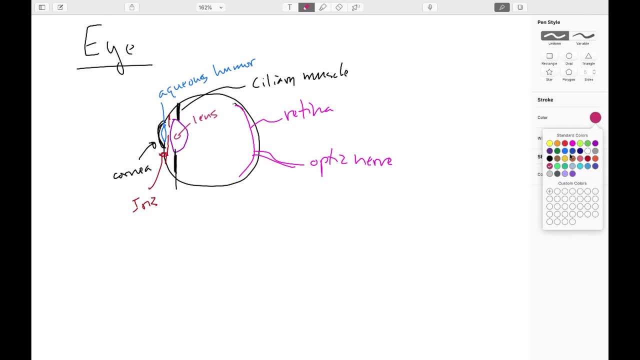 And by doing that, you can dynamically vary the focal length of the lens in order to bring things to a good focus. Now, to say good focus is stretching it a bit. It turns out that between the cornea, the aqueous humor- and the lens, it's a compound lens system all in contact with each other. 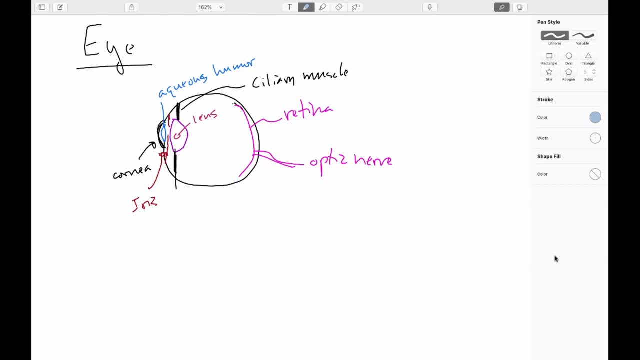 The bulk of the refraction occurs at the cornea. The lens is in contact with the cornea. The lens is responsible for adjusting things. It turns out the actual image quality cast on the retina is pretty lousy And the colors do not come to the focus at the same spot typically. 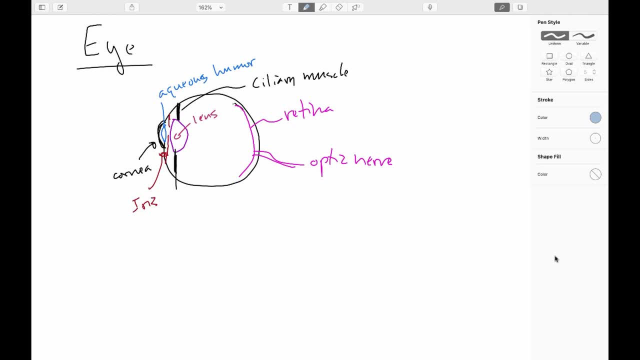 But it turns out that the brain does an awful lot of work to correct the image that is coming in on the retina And the colors do not come to the focus at the same spot typically. But it turns out that the brain does an awful lot of work to correct the image that is coming in on the retina. 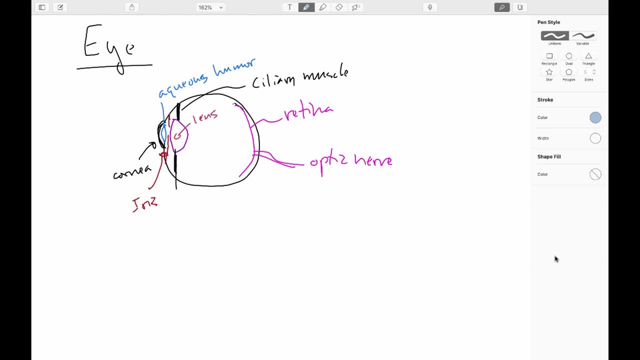 To give it the nice sharp images that we see. Thus, a lot of our optical illusions. Okay, So what could go wrong with the eye? Well, one thing that could go. Before we dive into talking about what could go wrong with the eye, let me define a couple terms real quick. 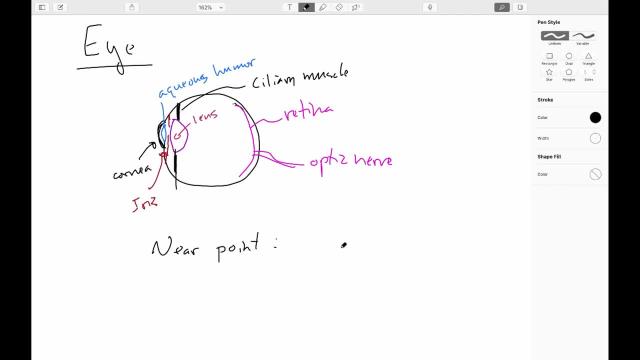 The near point of the eye is the closest distance you can focus. If you are, If you're a young person who hasn't had a lot of environmental stresses and all that, this distance is, too, Typically on the order of 25 centimeters. 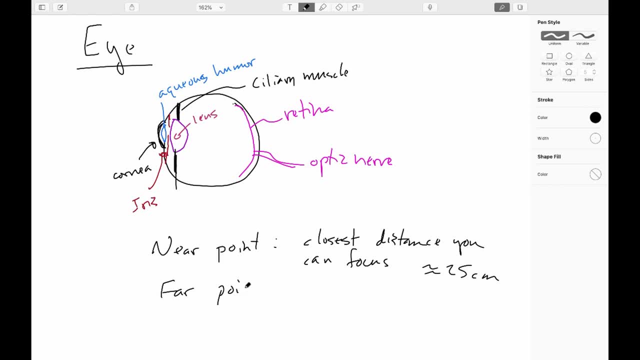 The far point is defined similarly. It's the farthest distance that you can focus. So again, for a young eye, that's approximately 3.8 million light years, the distance to the Andromeda Galaxy, Which is the furthest object that the unaided eye can see. 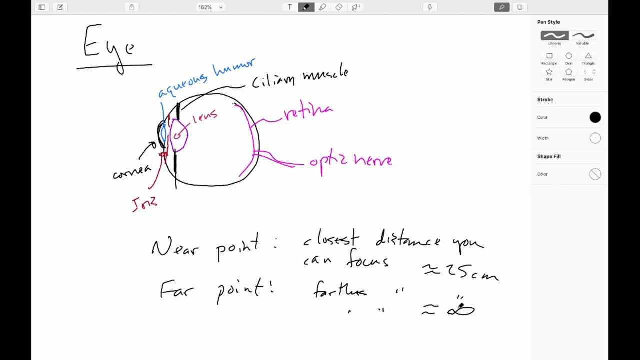 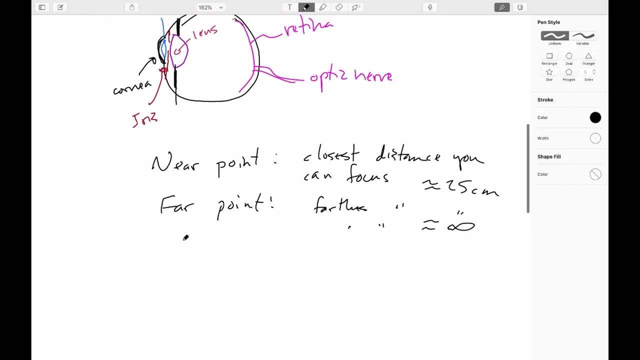 Let's just call that infinity and be done with it. So what can go wrong? So one condition you can have is what's called myopia, And the common English term for myopia is nearsightedness, And the thing to remember with that is that that's what works. 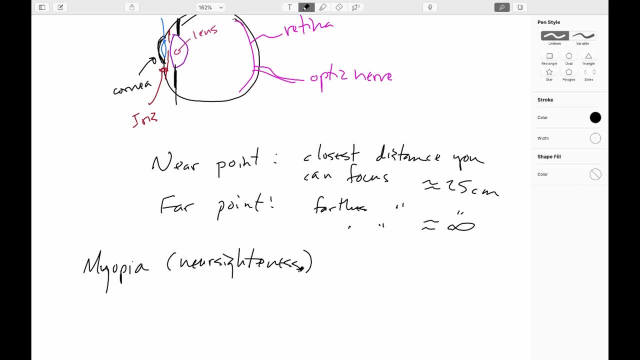 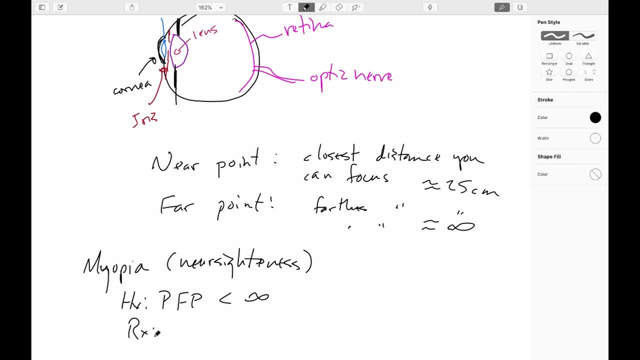 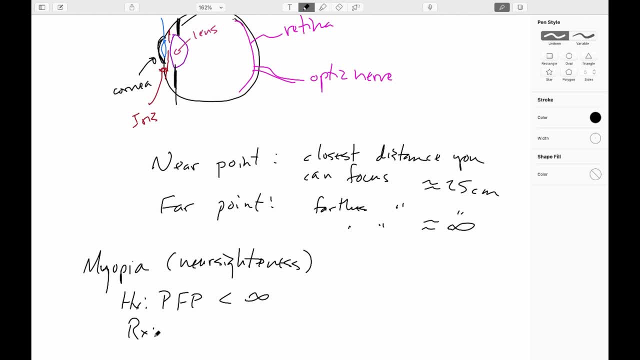 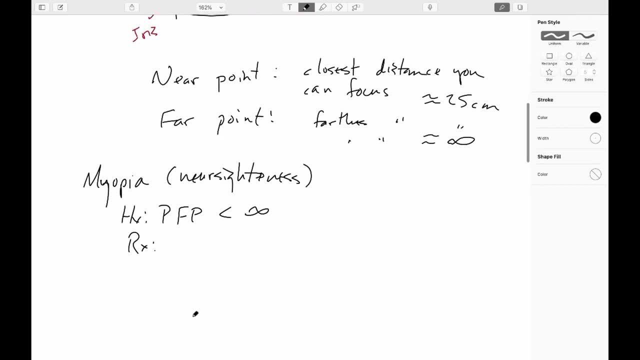 so so, so, so. so I won't bother doing eyeglasses, because the spacing between the glasses and the lens complicates things a bit. You would write a contact lens such that the choosing a focal, a focal length, such that the image distance would be equal to the negative of the patient's. 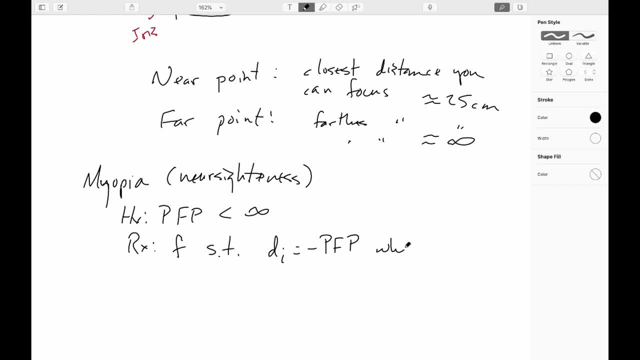 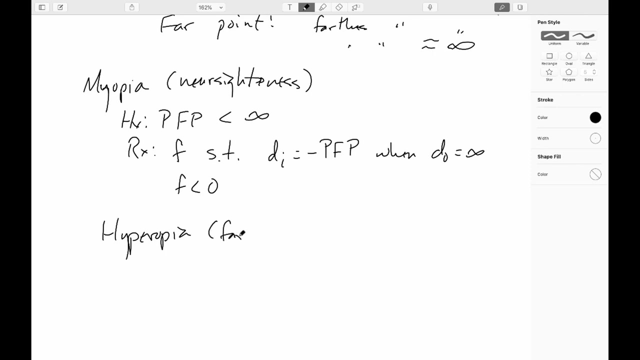 point when the object distance is equal to infinity, This will be a diverging lens, so f less than zero. Something else that could happen would be hyperopia, and these, both myopia and hyperopia- are usually due to the eyeball changing shape so that 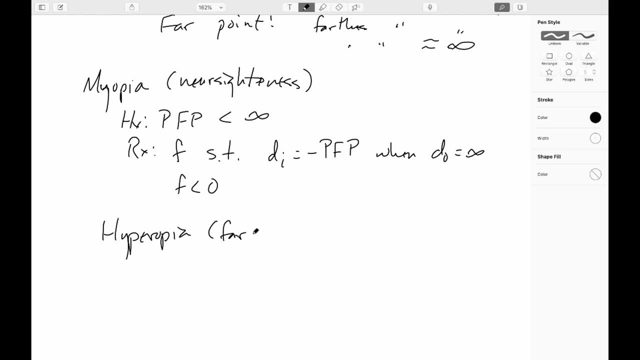 the retina isn't located where the lens can accommodate to. So here again, farsighted is what's working. So it's not working for the patient is that their near point is too far away. It's greater than 25 centimeters. So the prescription here would be to write a contact lens with a focal length. 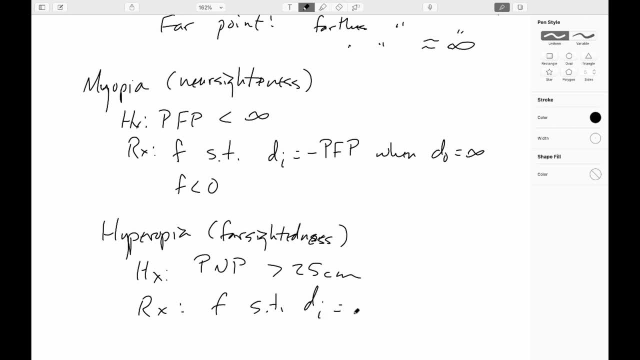 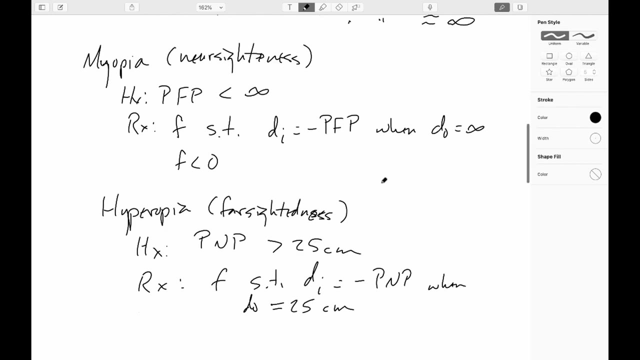 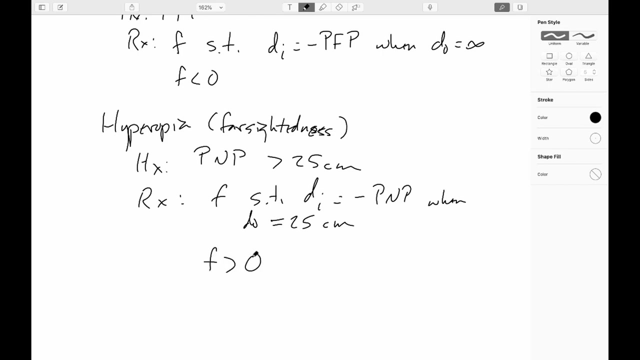 such that the image distance would be equal to the negative of the patient's near point when the object distance is 25 centimeters, And that will correspond to having a positive focal length, so a converging lens. So one way you can tell whether your glasses-wearing friend is nearsighted or farsighted is just. 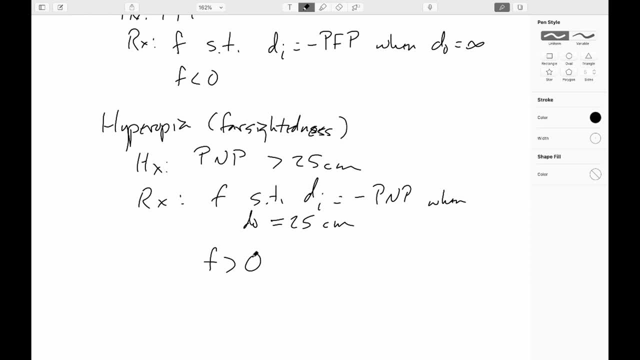 to look through their lens. If what you see looking through it looks shrunk down, then you know you have. that's a virtual lens. If it's a virtual upright and magnified situation, that would be case four. That would be a diverging. 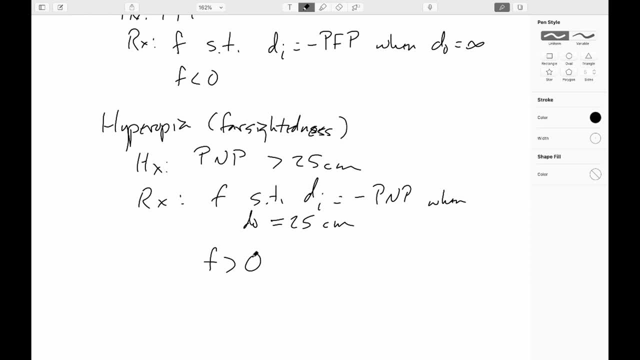 lens, and so they must be nearsighted. On the other hand, if you look through and everything looks magnified, then that would have to be a case three situation: virtual, upright magnified. That would be due to a converging lens, so you know that they would be farsighted. 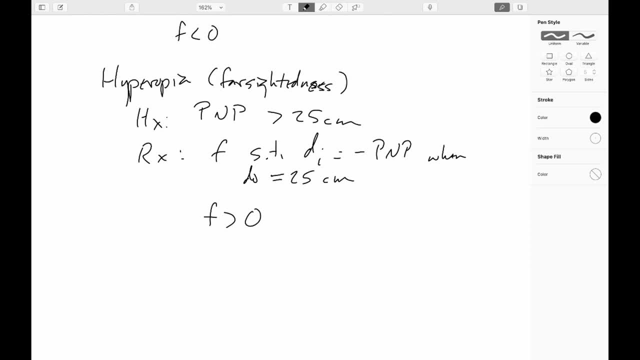 Added bonus would be: Um, If they, If they, If they have astigmatism. astigmatism means that the eye also has lost some of its spherical shape. so they fix that by putting some cylindrical curvature into the lens as well. 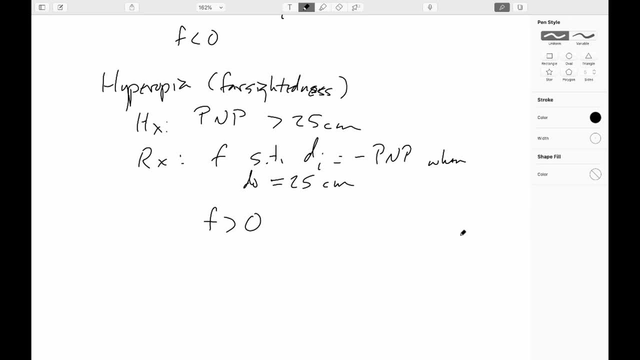 Some other things that can happen. probably my favorite named one is presbyopia, which, if you break the Greek roots apart, it literally means that thing: What happens to your eyes when you get old? What happens there is that the lens hardens, making it harder for the ciliary muscles to 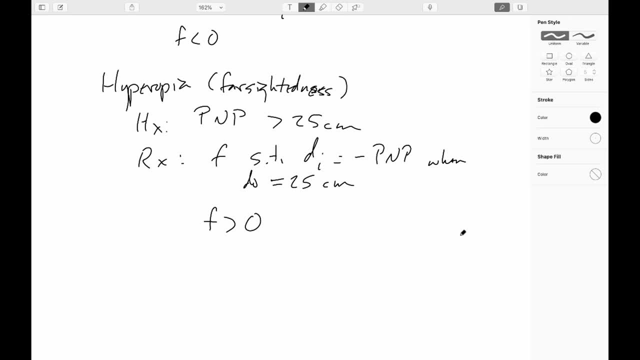 make the lens thinner. This has the result of pushing out the patient's far point. So what this winds up meaning is that you usually end up needing a prescription for every single distance that you want to look at. So either you're going to need reading glasses, or bifocals, or progressives, something like. 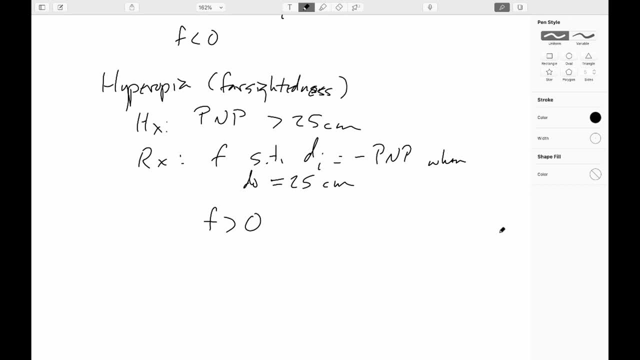 that. Other ones that you may have heard of include cataracts. There, the issue is that the lens is becoming opaque. This is usually due to ultraviolet light denaturing some of the proteins that make up the lens. The resolution for that is to do a surgical procedure where you replace the lens with 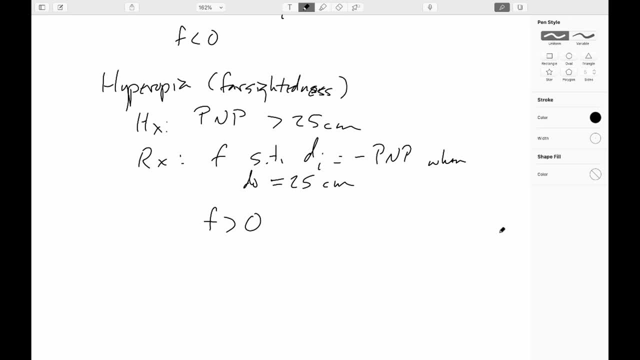 a surgical procedure. Okay, So you may have heard of a prosthetic plastic lens and you may have heard of glaucoma There, the vitreous humor, which is the fluid that is between the lens and the retina. the pressures can get to be too high and cause the nerves to die. 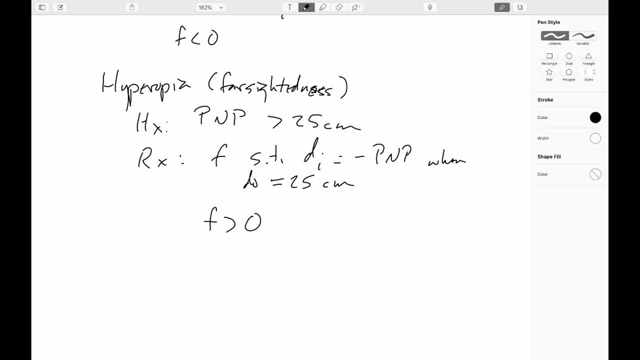 Okay, So the reason why glaucoma is so vicious is because the retina is thinner out at the edges. It's quite possible to not realize that you're losing your vision because the field of view is shrinking slowly from the inside. So this is why, if you've ever gone into the eye doctor and they've done that thing, where they blow the puff of air on your eyes Or they stick a I don't know. I don't know. They stick a device literally right on your eye where you see like a scary blue ring of light. What they're doing is they're measuring the pressure in the eye to see if they need to. 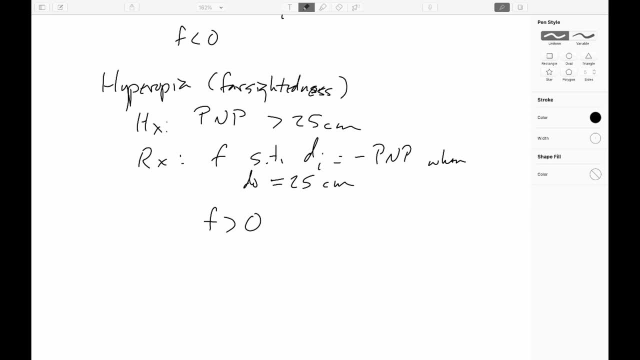 start to prescribe drugs to correct for that. Anyway, let's just do a quick example of this. Let's say you have- Okay, Okay, Okay, Okay. Let's say you have- a patient who is hyperopic, Okay, And their near point is 60 centimeters. 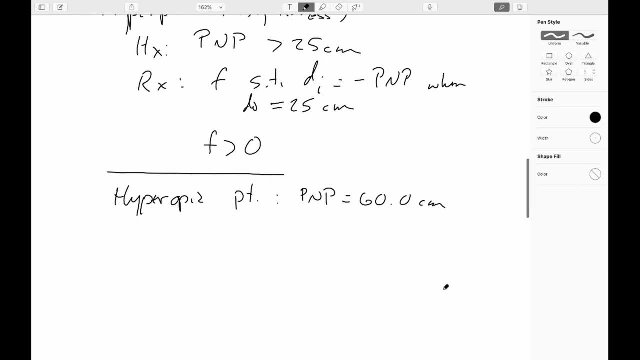 So remember hyperopia. Hyper means far Right. By the way, E antenna is hyper. it's about five centimeters, Very, very far. That means that what works for them is seen far away. What doesn't work for them is what's up close. 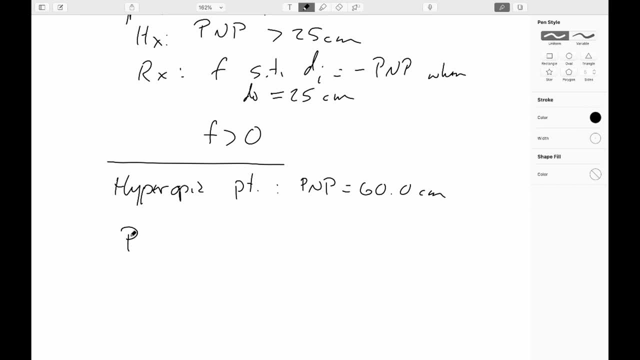 So usually what we want is the refractive power of the lens. So the nice thing here is that that's solving for 1 over f, So you can just plug straight in the most useful equation in optics, As long as we set up our dO and our dI correctly. 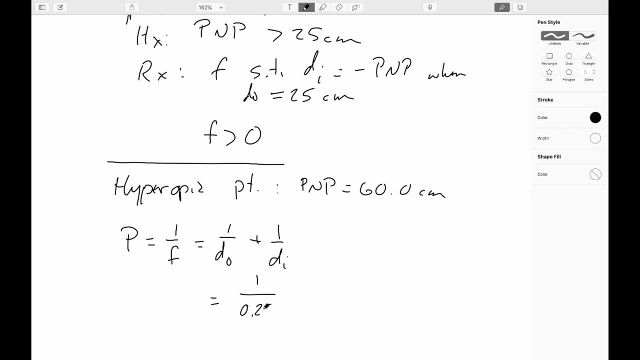 So dO here would be 0.25 meters- That would, because that's the where we would like our object to be, to match the young eye- And dI would be negative 0.60 meters, And that's because that's we want to park a virtual image out at the patient's near point in order to correct. 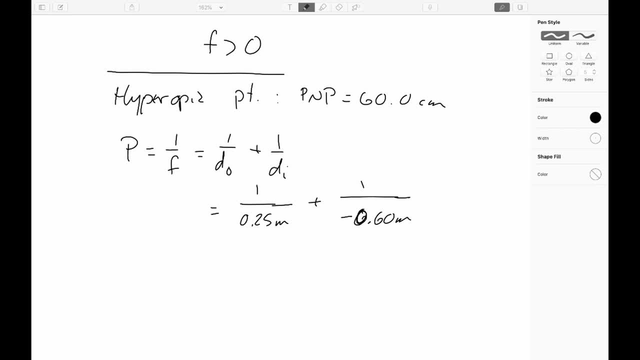 So we can go ahead and grind that through And get that. the patient should receive a plus 2.3 diopter lens. If we are doing contact lenses Now as a practical matter, they're probably going to be written for either like 2.25, 2.5, something like that.